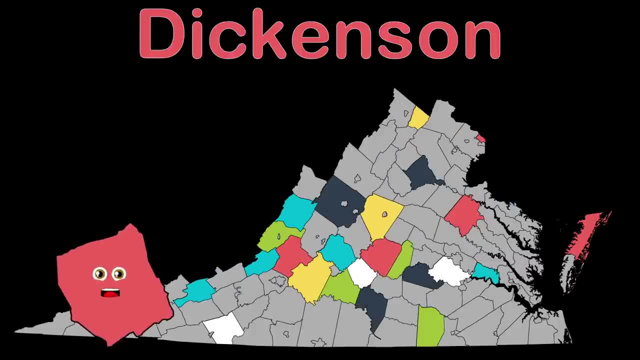 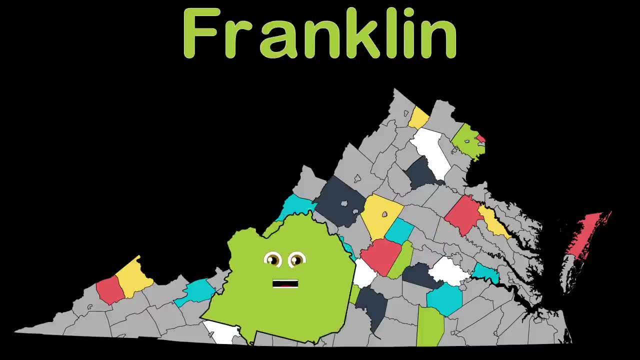 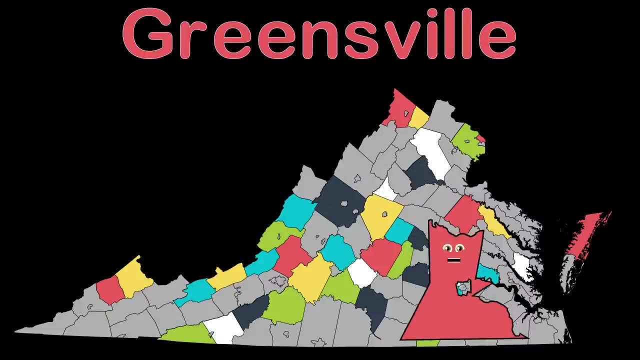 Craig, Culpepper, Cumberland, Dickinson, Dinwiddie, Essex. Fairfax will win: Fauquier, Floyd, Fluvanna and Franklin, Frederick Giles, Gloucester and Goochland, Grayson, Green, Greensville and Halifax, Hanover, Enrico Henry, Highlands on track. 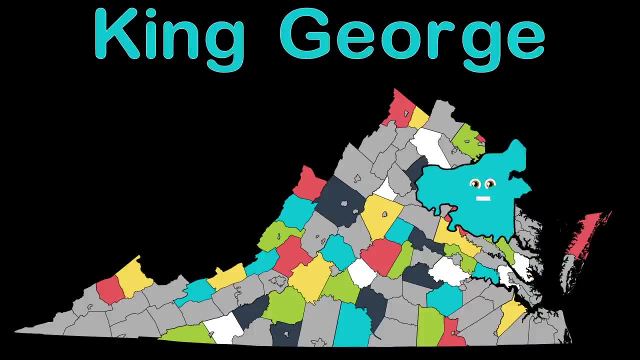 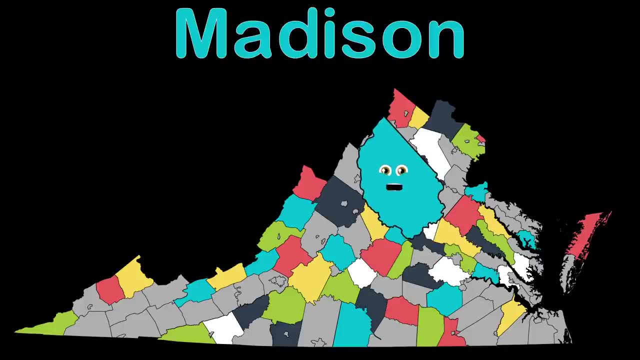 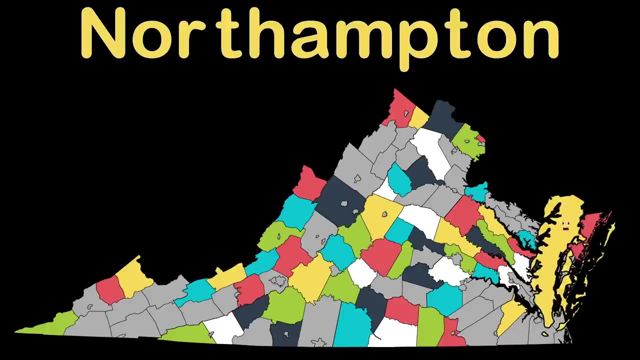 Isle of Wight, James King and Queen, King George, King William, Lancaster, Lee, Loudons Forge, Louisa, Lunenburg, Madison, Matthews, Mecklenburg, Middlesex, Montgomery, Nelson Strew, New Kent, Northampton, Northumberland, Nottoway, Orange Page Patrick. 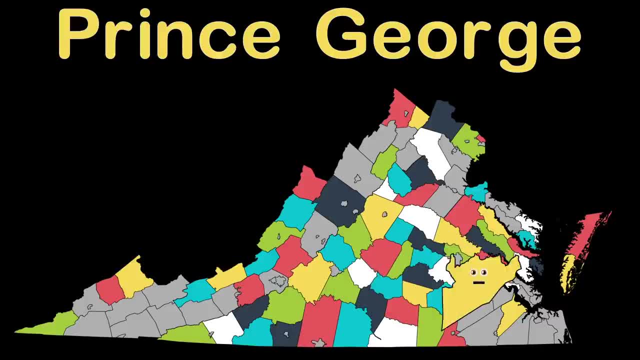 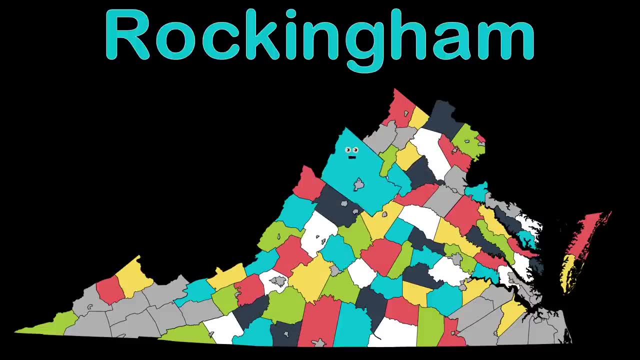 Umar, Pennsylvania's way: Powhatan, Prince Edward, Prince George, Prince William, Pulaski, Rappahannock, Richmond, Roanoke, Rockbridge, Rockingham, Russell, Scott just woke- Shenandoah Smith, Southampton. 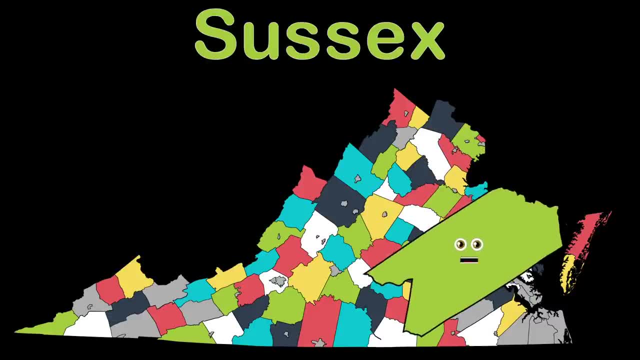 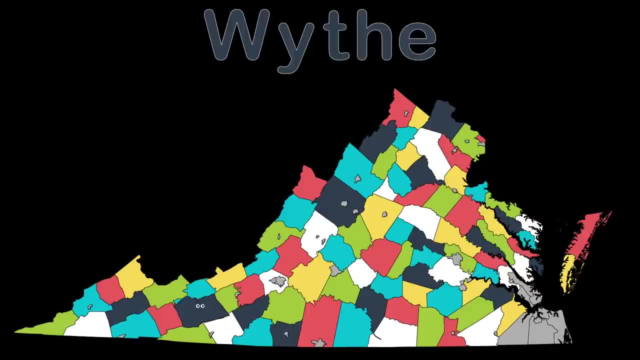 Spotsylvania, Thaford, Surrey, Sussex, Tazewell, just sawya, Lauren, Washington, Westmoreland, Wise, Wythe, York. there's more, don't be surprised. We're the Magic. Here's our team show Most with most percentage. whoop Dies السمensional deus או سך. Feliz que Jesus tenemos a todos cuál. We're the Magic. Here's our team show Most with most percentage. whoop Dies 가서 Wahr and Feliz que Diosatan. todos os aconch Qu laughing Valeromoreましょう, ficou iguales wieder que vimos. welítulo l railroadишь que un pastor no esР. 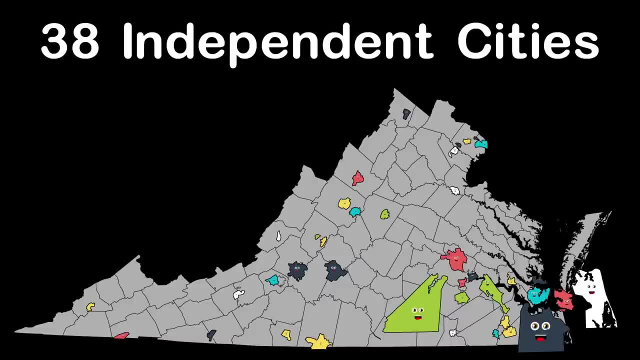 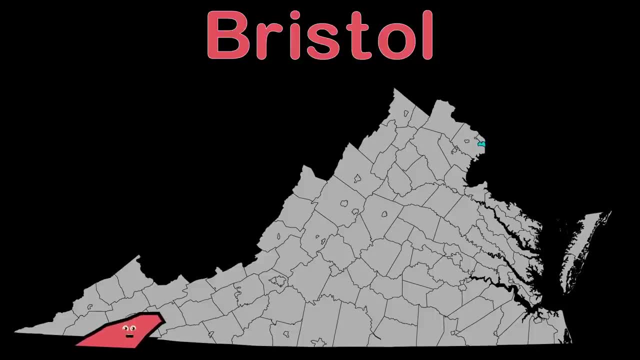 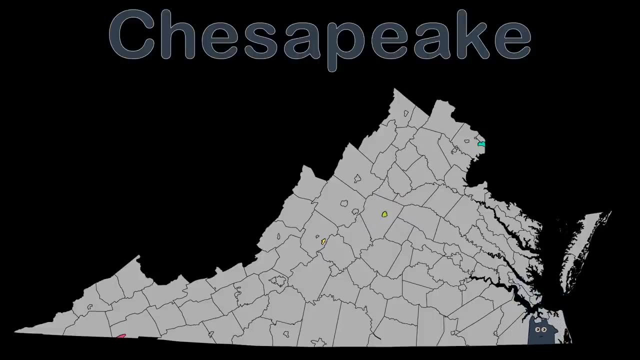 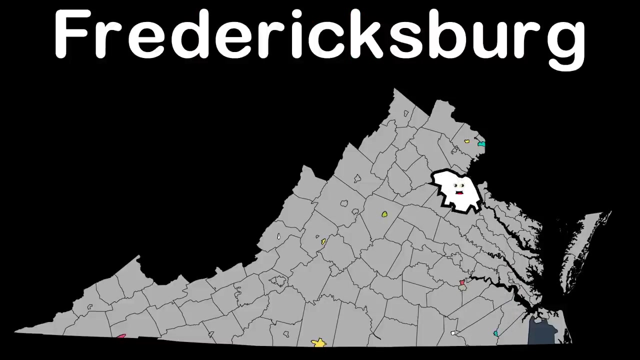 The 38 independent cities you'll learn Now. please pay close attention, because it is our turn. Alexandria, Bristol, Buda Vista And Charlottesville, Chesapeake, Colonial Heights, Covington, I'm Danville, alright, Emporia, Fairfax, Falls Church, Franklin's intact, Fredericksburg, Galax, Hampton. 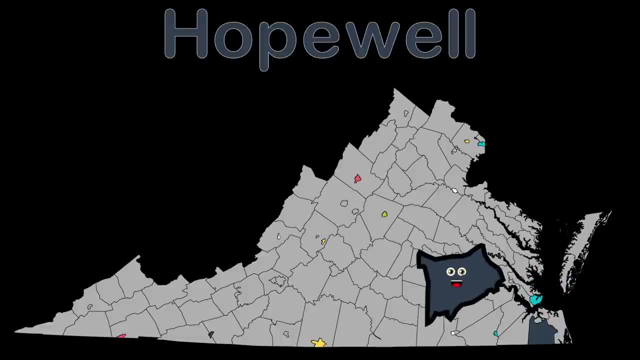 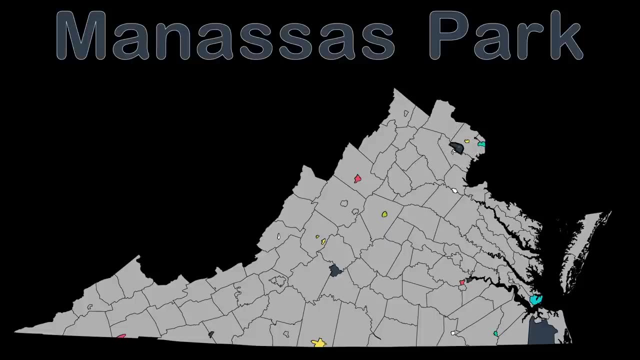 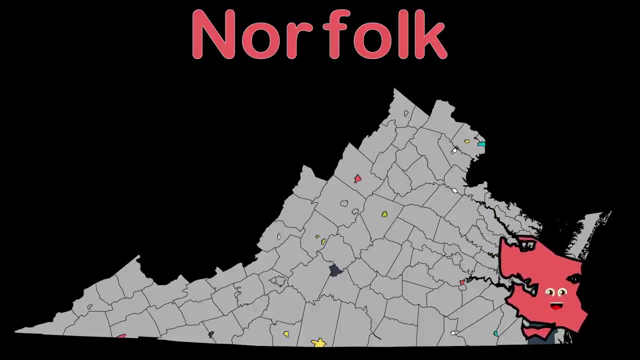 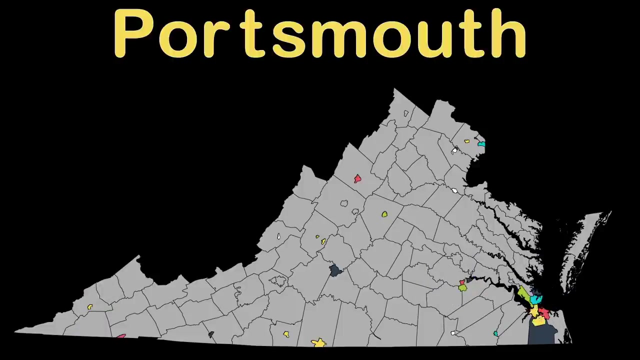 I'm Harrisonburg, that's a fact. Hopewell, Lexington, Lynchburg, Manassas is on track. Manassas Park, Martinsville, Newport News, Norfolk, it's a thrill. Norton, Petersburg, Pocosin, Portsmouth, just like you heard, Radford, Richmond, Roanoke And Salem isn't blurred.